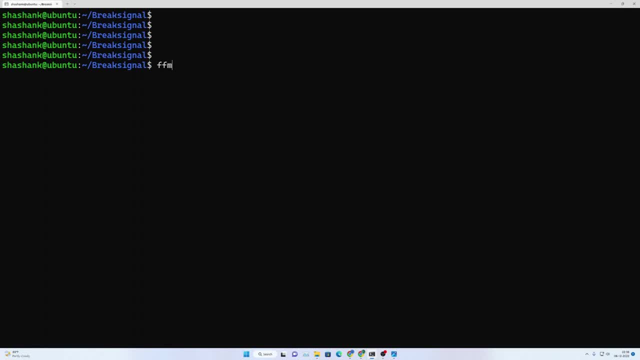 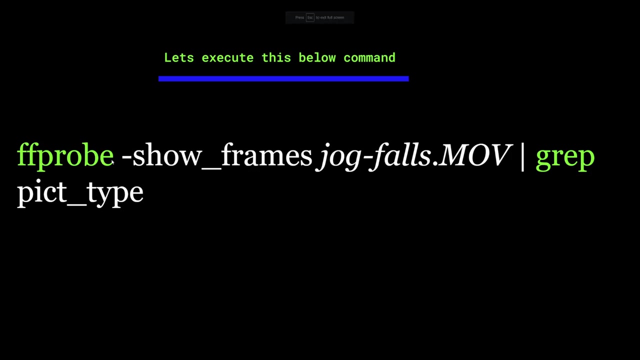 Now. so, if you see, I have installed FFmpeg on my computer and so also I have the video here, jokefalsemov. So let's quickly first examine the command that I have over here. We will be using an FF probe. Basically, it would have been installed when you installed. 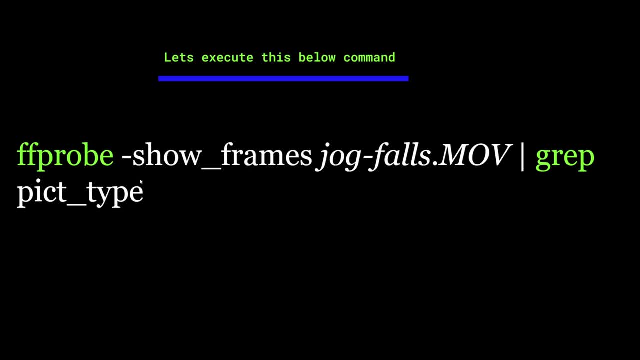 FFmpeg. So we will be going through a list of frames and also, once we get the list of frames in this video, we will be interested in what type of frame it is, or you can say what type of picture it is, A picture type you can say. So to do that, let me first quickly execute this command. 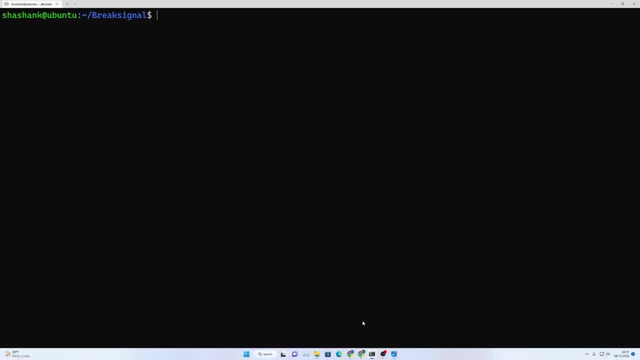 over My terminal. So when I enter this, you see I'm going to stop it here. If you see there is an picture type i or you can say frame type i, There is frame type b and there is frame type p, So let us try to find more and know. So these three are the major ones that I can see here. 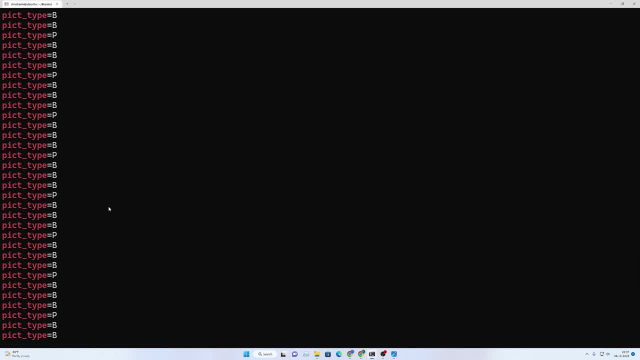 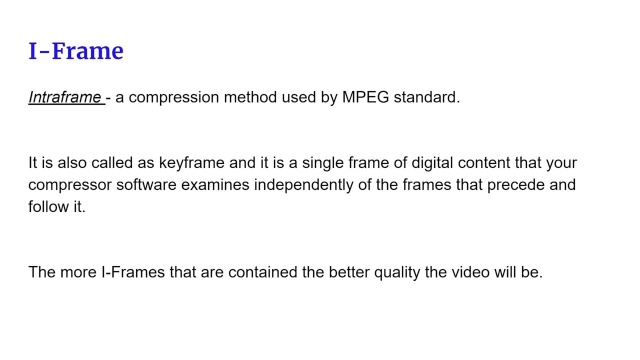 So what are these types? What are these frames? I frame, B frame and a p frame. So what is I frame and why is this frame So important? Iframe We can call it as an intra frame or you can call it as a leader frame. It is used as a 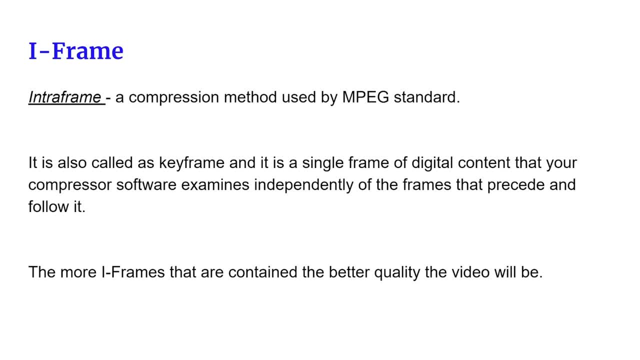 compression method by MPEG standards. Now, this frame: it contains all the data Like how, What is the compression algorithm and what, And all theife is a friend should be represented. So it contains all the data. So the compressor software that I use for most of the work in this particular 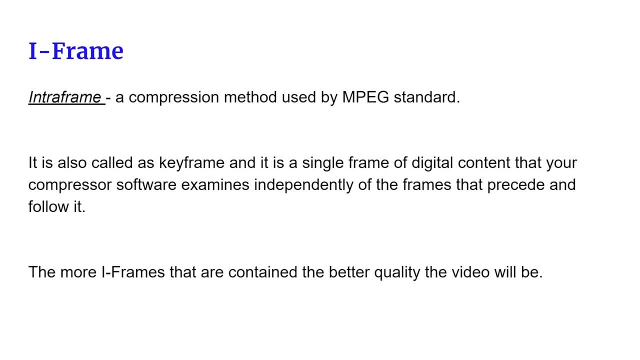 compressor software or the compressor algorithm is interested in reading this frame. It won't read this B frames or it won't read this P frames. it is interested in this intra frame because it has the information how the frame should be represented, how the frame should be decompressed. 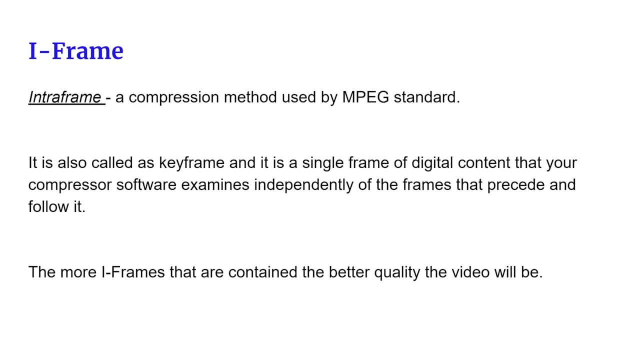 or decoded and should be represented. So that's why I frames are also called as leader frames. Another important factor is the more number of iframes, the better the quality of the video. Okay, so if you see in the previous example that I showed you, there were multiple iframes in